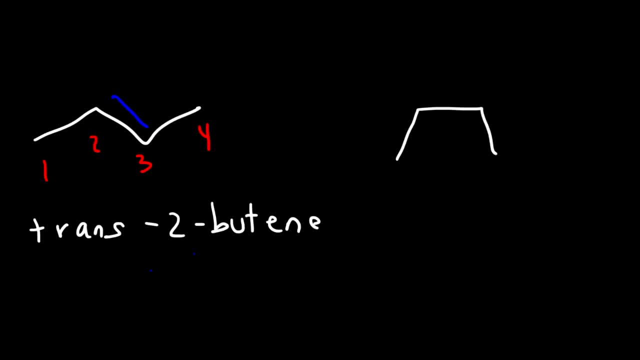 you want to be specific, And then this structure here is cis-2-butene. Go ahead and name this one. So what's the name for that particular alkene? So 1, 2, 3, 4, 5, 6,, 7.. There are seven carbons and we have a doubled bond at 2 and at 5.. So this is going. 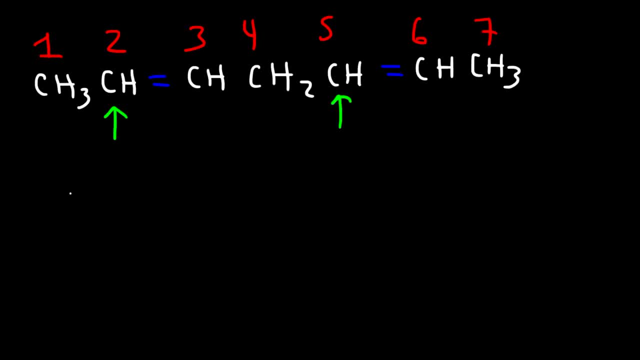 this is going to be a dying. so this is two comma five, and because the seven is going to be heptane, we could say heptadien. now, what about this one? let's say, if we have a methyl group, how can we name this particular alky? so we: 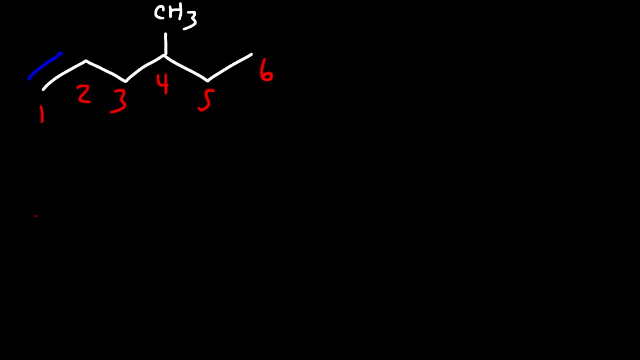 need to give the double bond the lower number. so we need to put a carbon one. so this is going to be for methyl one and we have six carbons in the longest chain. so that's hexane, but it's going to be. one vaccine is another one that you 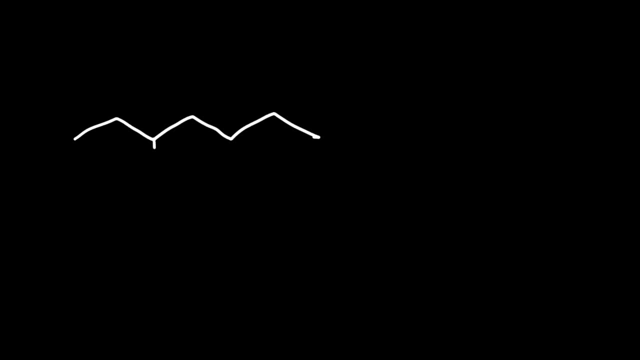 could try. so let's say we have a chlorine atom, a bromine atom and a double bond. so go ahead and try that. so this is going to be carbon one, two, three, four, five, six, seven. so we need to count in such a way that we give the double bond priority. we 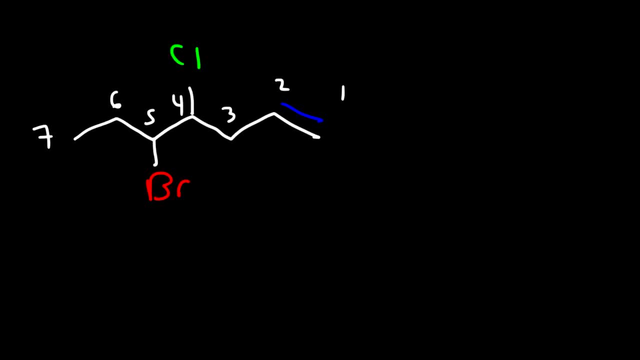 give it the lower number. we still have to put in alphabetical order. we have a five, bromo, and we have a chlorine on four. so that's a four chloro and we have seven carbon. still, instead of saying heptane is going to be heptane and there's a double bond at carbon one. so putting it all together, 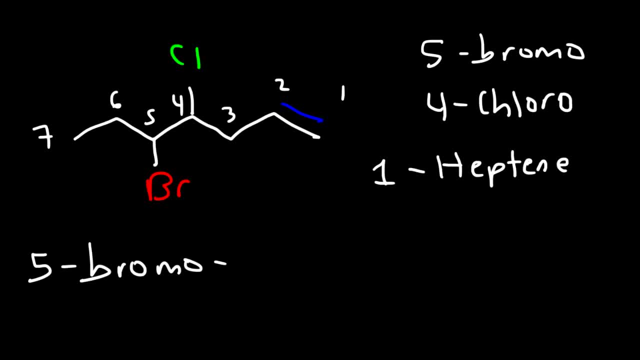 it's going to be five bromo dash, four chloro dash, one heptane, and so that's how we can name this particular molecule. now let's move on to the next problem. so how can we name this particular alkyl? what is the longest chain? so, looking at the structure, it appears that 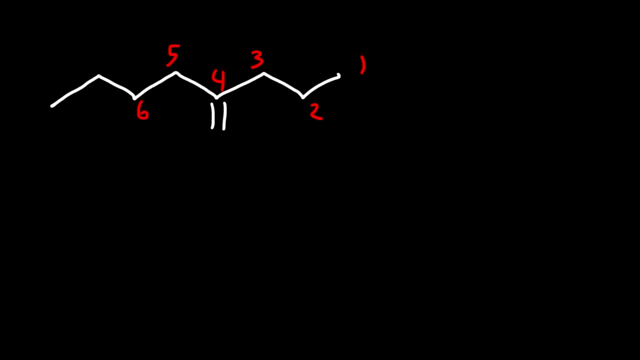 this is the longest chain. we have eight carbon atoms. the only issue with this chain is that it does not include the functional group, the alkyl, so we can't use it, even though it's the longest chain. so therefore, this is going to be the longest chain because it includes the 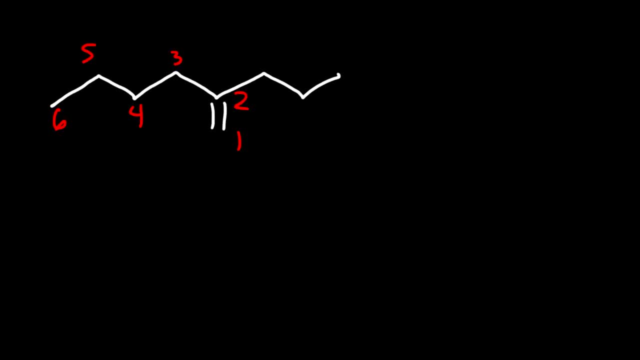 alkyl. so we have a six carbon chain and the double bond is between carbons one and two. so this is going to be one hexene attached to carbon two. we have a propyl group. there's three carbons here. so we're going to say this whole thing. 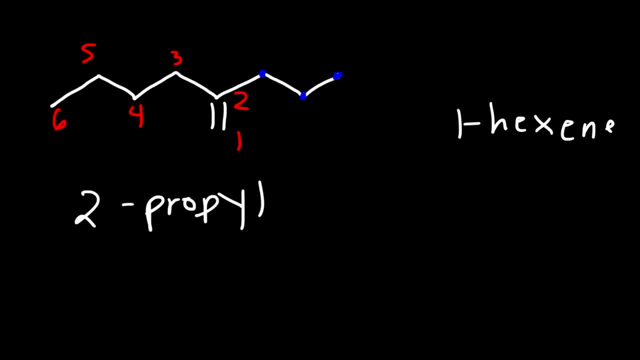 is two propyl dash, one hexene, so you need to include the alkene functional group in the longest chain. now let's try some examples with cycloalkenes. so try these two examples. so the first one has five carbon atoms in a ring, so that's a cyclopentane ring, but with the alkene. 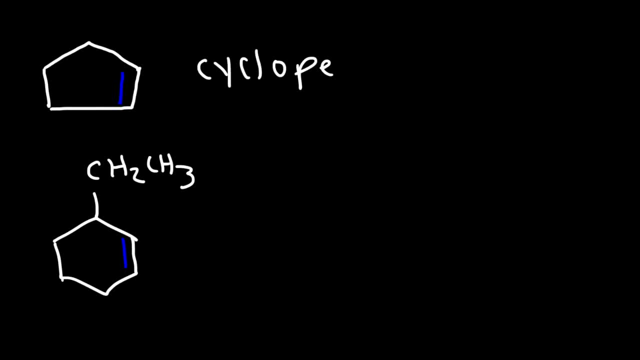 it's going to be called cyclopentene. now the one below it. we have a six carbon ring, so it's going to be cyclohexene, and then we have an ethyl group. so what is the number that is associated with the ethyl group? we can't count it this way. 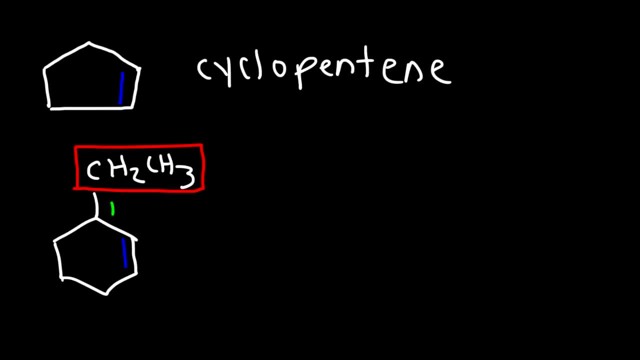 because we need to give priority to the alkene. so automatically the alkene is going to be on carbon one, so this should be called 3-ethyl-cyclohexene. let's consider another example. so let's say we have a methyl group and a bromine atom attached to the ring. 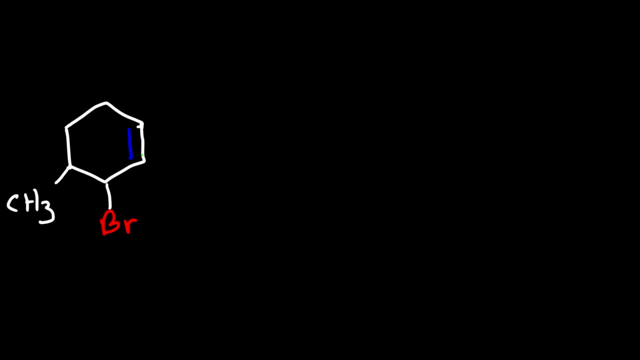 go ahead and name this particular cycloalkene, so this has to be carbon one, two, three and four, so this is called 3-bromo, because we need to put it in alphabetical order: dash 4-methyl and then, after that, cyclohexene. 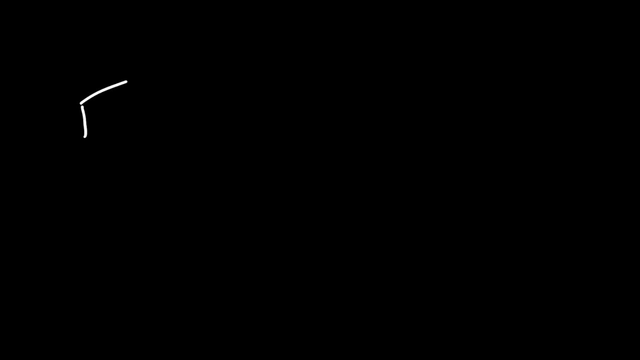 let's work on one more example. so how should we name this particular alkene, and which is the best way to count it? so if we count it this way, the ethyl group will be on carbon five and the methyl group will be on carbon six, but if we count it the other way, the 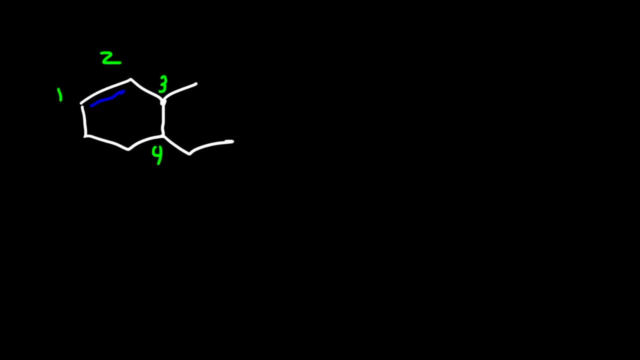 methyl group is on carbon three and the ethyl group is on carbon three and the ethyl group is on carbon six. Let's compare that by adding these two numbers together. group is on carbon 4. So we get lower number substituents. So ethyl comes before. 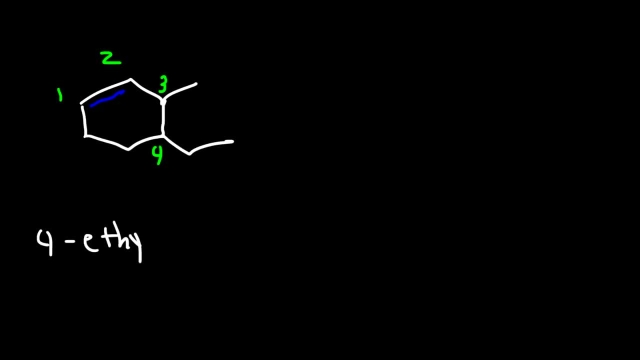 methyl. so it's going to be 4-ethyl-3-methyl and then cyclohexene. So that's the answer. Now let's go ahead and move on to E and Z isomers. So feel free to pause the video and determine if this molecule represents the E isomer or if it. 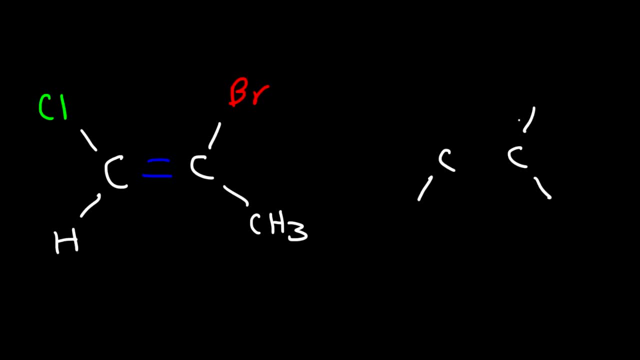 represents the Z isomer. So what do you say about the compound on the left? Do we have the E isomer or the Z isomer? So we need to identify the highest priority attached to each carbon of the double bond. So let's focus on 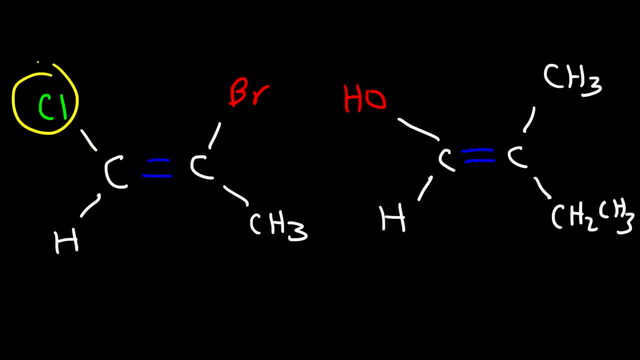 this carbon. So, comparing chlorine and hydrogen, which one has a higher priority? Chlorine has a higher atomic number, so this is going to be the highest priority group. So between these two, which one has a higher priority? It's definitely going to be Br. Now, when the two highest priority groups are on the same side, you. 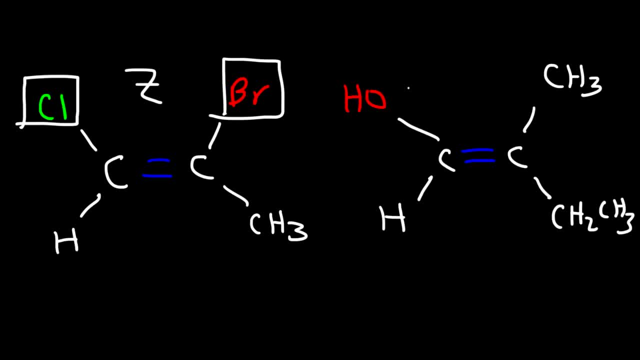 have the Z isomer For the compound on the right. comparing the hydroxyl group with hydrogen, the OH group has more priority, And comparing the methyl group with the ethyl group, the ethyl group has more priority, And so when the highest priority groups 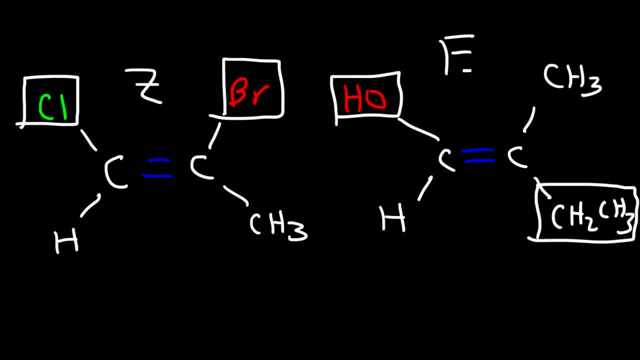 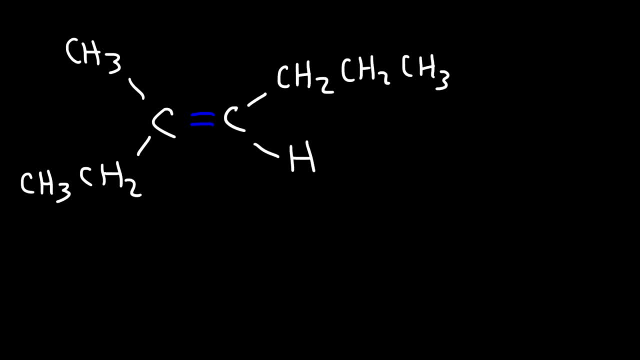 are on opposite sides, then you have the E isomer. Now let's work on this problem, Go ahead and identify if we have the E or Z isomer and name the compound. So if we look at these two groups, we can see that the ethyl group has more priority. 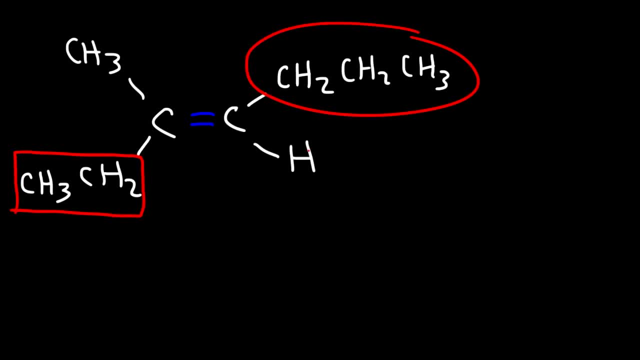 than the methyl group And comparing these two groups, the propyl group has more priority than the hydrogen. So, because the highest priority groups are on opposite sides of the alkene, we have the E isomer. So how can we name it? 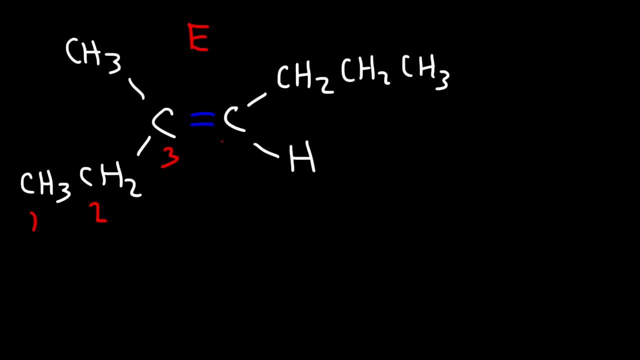 Well, we need to count the carbons: Carbon one, two, three, four, five, six, seven. So we have a seven carbon chain. This is going to be heptene, with the double bond at three, And we have a methyl group on carbon three. So first we need